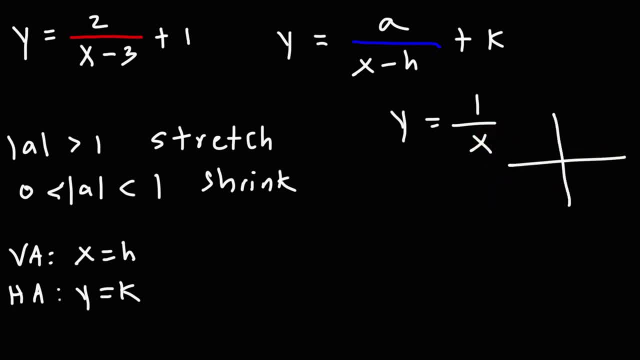 y equals 1 over x. This graph has a generic shape that looks like this: When a is positive, when it's greater than 0, the graph is going to exist in quadrants 1 and 3.. Now, when a is negative, let's say if we have y equals negative 1 over x. 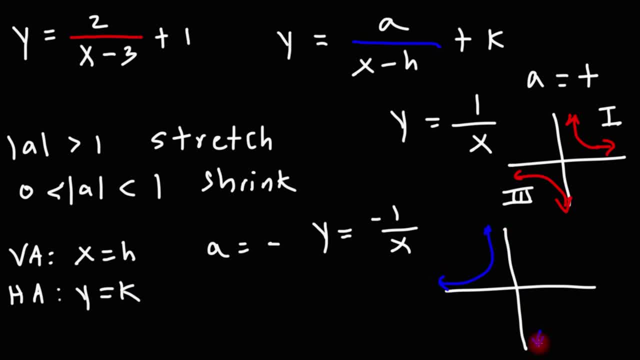 the graph is going to exist in quadrants 1 and 3.. The graph will exist in quadrants 2 and 4.. So this is quadrant 2, this is quadrant 4.. So those are some things you want to know when graphing reciprocal functions. 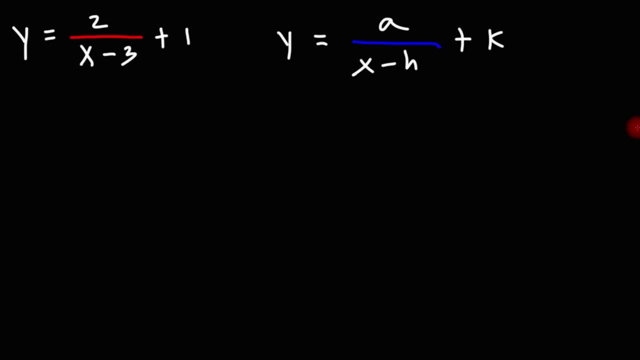 which are the same as rational functions or very similar to it. So let's focus on this particular reciprocal function. We can see that h is 3, k is 1.. So the vertical asymptote which is x is equal to h. it's going to be x is equal to 3.. 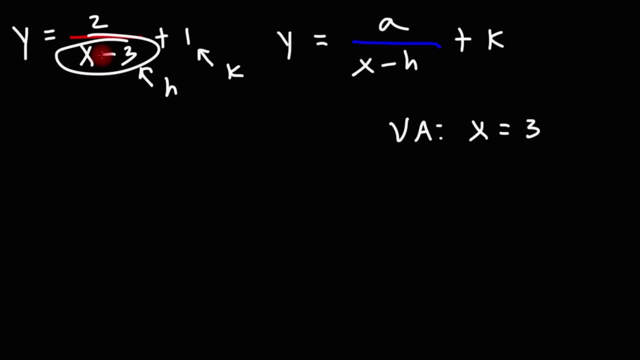 If you set x minus 3, equal to 0, and solve for x, you'll get x is equal to 3.. For the horizontal asymptote, it's simply: y is equal to whatever number we see here. So in this case it's going to be: y is equal to 1.. 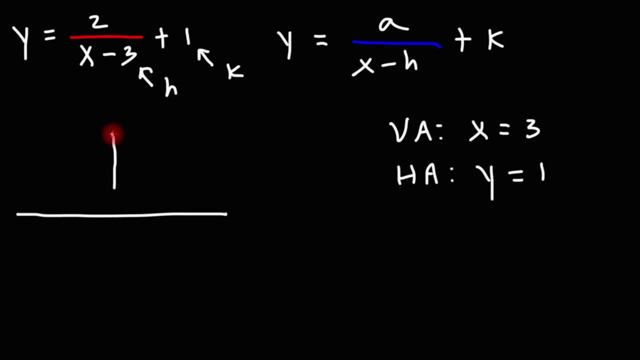 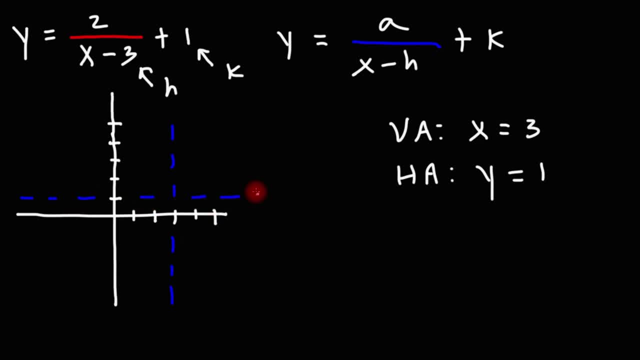 So at y is equal to 1, we're going to have a vertical asymptote. So at y is equal to 1, we're going to have a horizontal asymptote. Now, if all we wanted was a rough sketch of the graph, 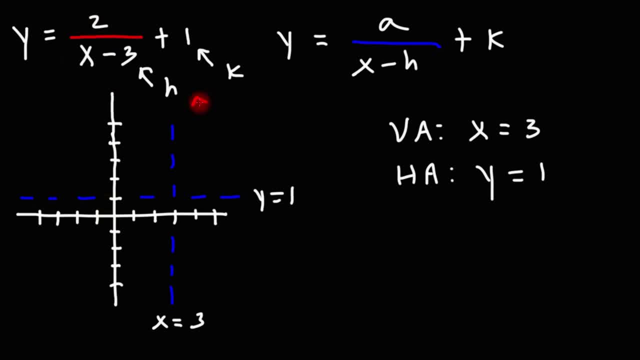 because A is positive, we know the graph will be in this quadrant. and in this quadrant, That is, the quadrants defined by the horizontal and vertical asymptotes, not necessarily by the x and y axis. But to get a more accurate graph, what we can do is we can plot a few. 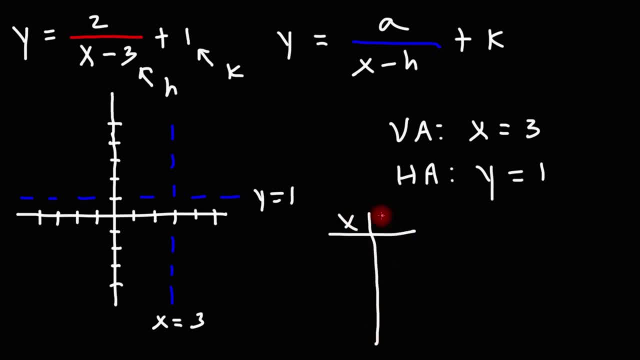 points. So I'm going to pick an x value, one unit to the right of the vertical asymptote, So I'm going to go with x equals 4.. And also one unit to the left of that And x equals 2.. 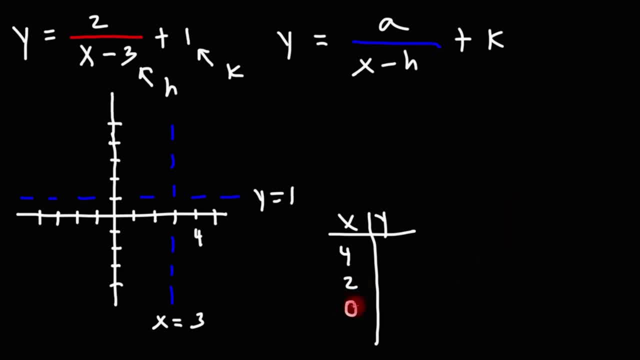 And I also want the y intercept, so I'm going to use 0 as well. So plug in the numbers into this equation. Starting with 4, we have: y is equal to 2 over 4 minus 3 plus 1.. 4 minus 3 is 1.. 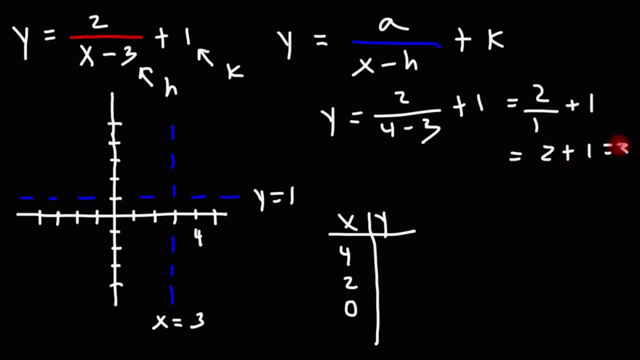 2 over 1 is 2.. So 2 plus 1, we get 3.. Now if I were to plug in this, I would have to plug in the x value. So if I were to plug in 0, I mean x equals 2,. 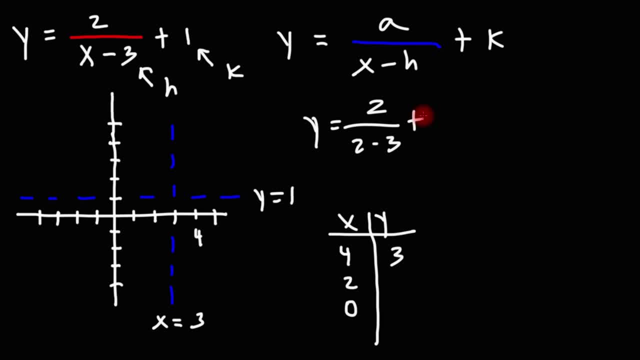 we would get this. So 2 minus 3 is negative 1. 2 over negative 1 is negative, 2. Negative 2 plus 1 is negative 1. Now let's get the x intercept. Let's replace x with 0.. 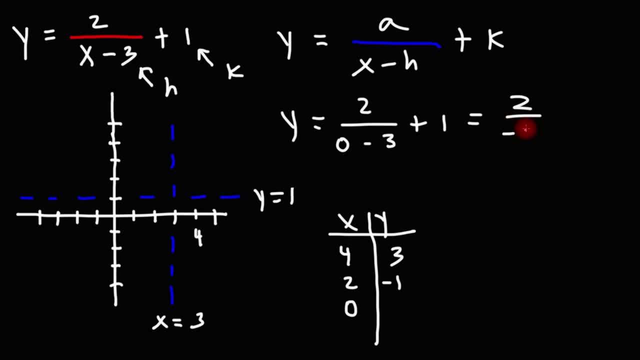 And I forgot about the plus. So this is 2 over negative 3 plus 1.. We can replace 1 with 3 over 3.. 3 divided by 3 is 1. Negative 2 over 3 plus 3 over 3 is: 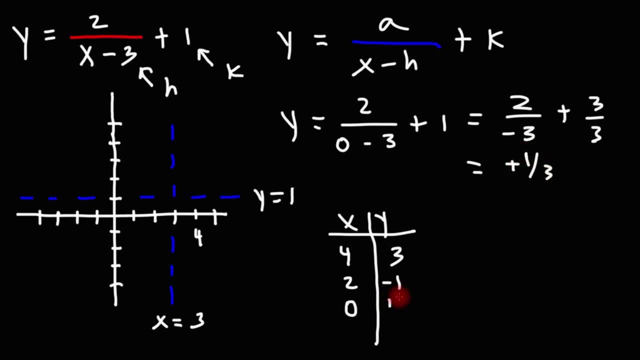 positive, 1 third. So, plotting these points, we have: x is 4, y is 3.. So we have a point there: When x is 2, y is negative, 1.. And when x is 0, y is 1 third. 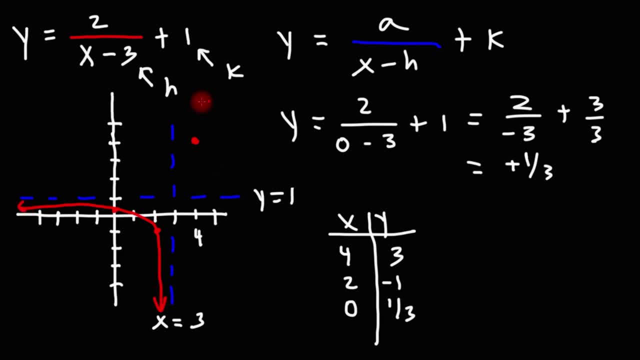 So we can replace 1 with 3 over 3. And we can draw a more accurate sketch with this. Of course you can add more points to make it even more accurate, But that's a rough sketch of this particular reciprocal function. 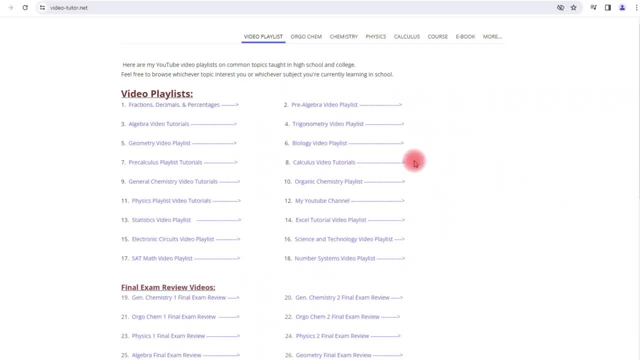 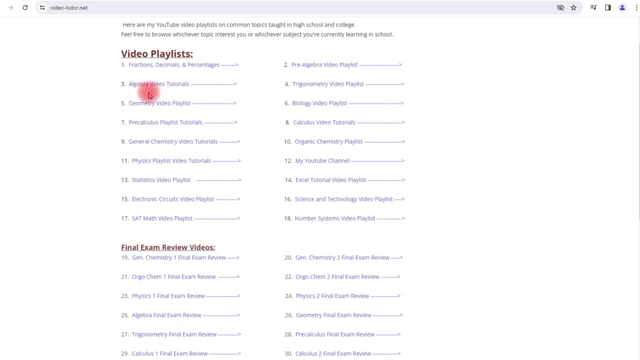 For those of you who want to quickly access my math and science video playlist, feel free to check out the website video-tutornet. You'll find playlists on algebra, geometry, trigonometry and algebra, And I'll see you in the next video. 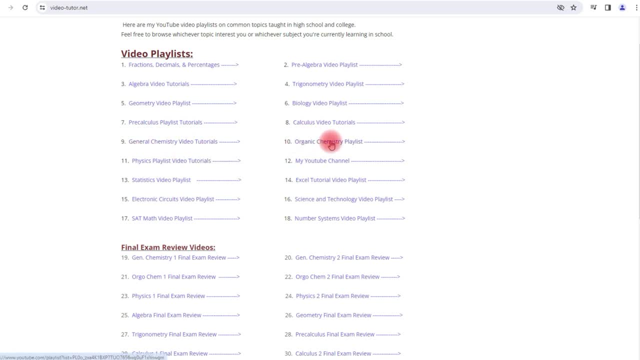 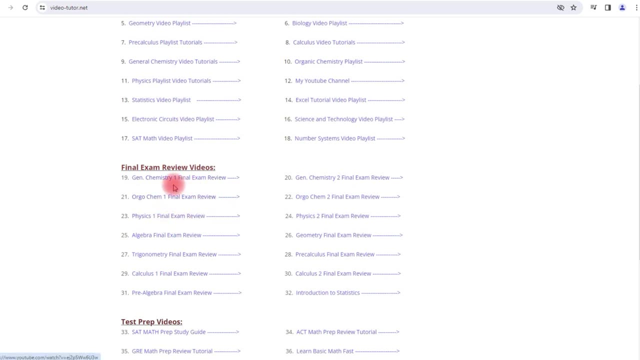 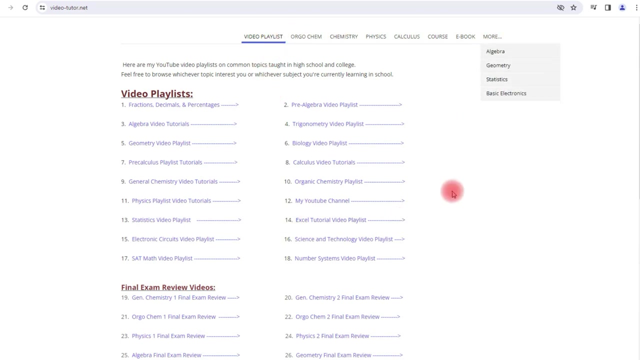 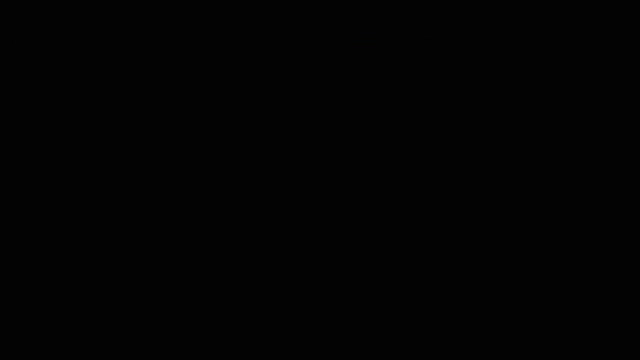 Thank you for watching. Reciprocal function y is equal to negative 4 over x plus 1 plus 2.. Feel free to pause the video if you want to try this example. So let's identify the horizontal and the vertical asymptotes. 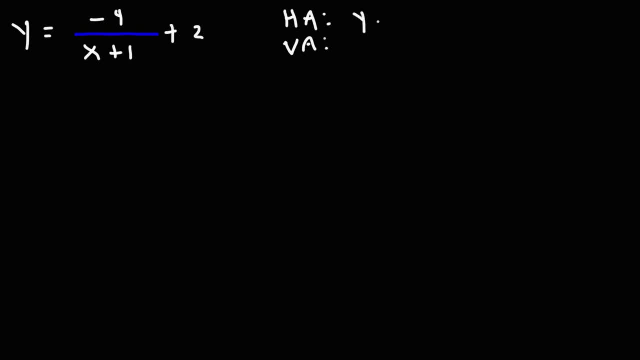 So we can see that our k value is 2.. So the horizontal asymptote is going to be: y is equal to 2.. For our vertical asymptote we're going to use the horizontal asymptote. For our vertical asymptote, if we set x plus 1 equal to 0 and solve for x. 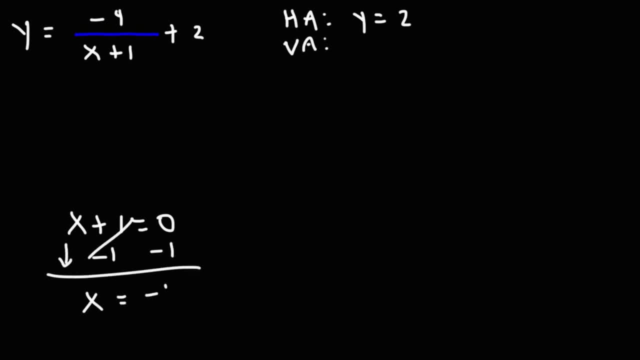 we're going to get our h value, which is negative 1. So the vertical asymptote is: x is equal to negative 1.. With this information we can go ahead and graph the reciprocal function. So we have the vertical asymptote at negative 1.. 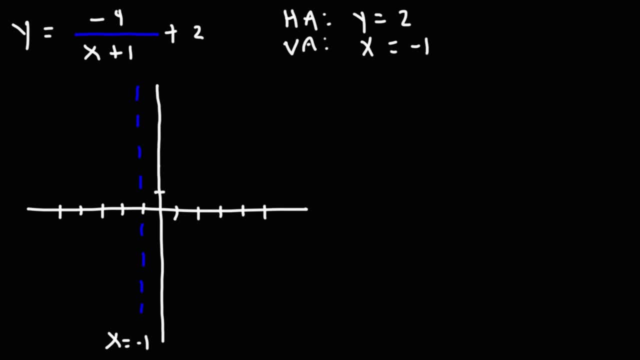 And we have a horizontal asymptote at 2.. First I need to put this in: So at y equals 2, we have our vertical asymptote. Now we do have a negative sign in front of the 4.. So we know the graph is going to look something like this: 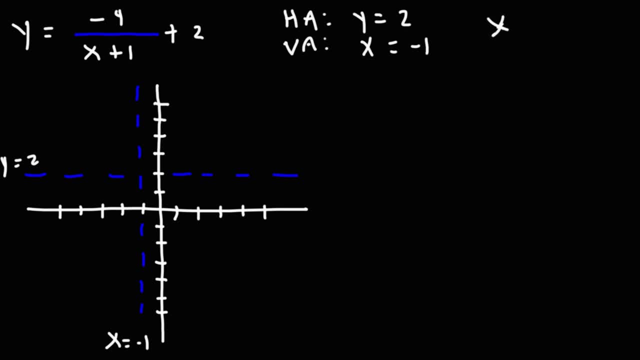 Now let's go ahead and make a table. So let's pick one number to the left of the vertical asymptote. I'm going to try negative 2.. So plug in negative 2 into the original formula. We'll have this: 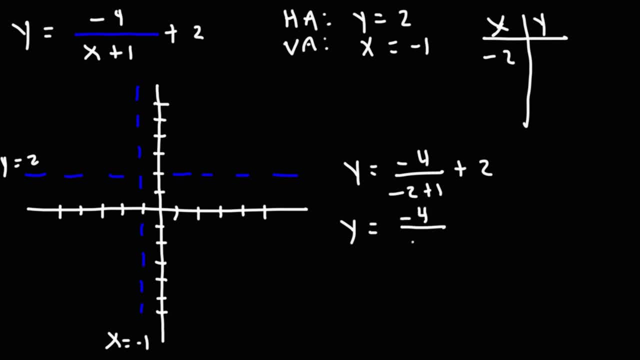 Negative 2 plus 1 is negative 1.. Negative 4 divided by negative 1 is positive 4 plus 2. That will give us 6.. Now we can also get another point to the left of the vertical asymptote. 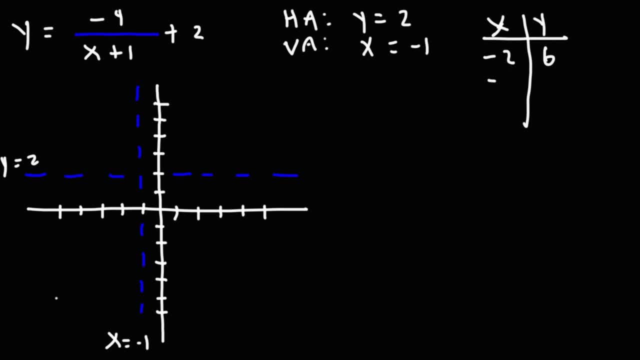 So if we try negative 1. Actually, we can't try negative 1. Let's try negative 3. If we plug in negative 3, negative 3 plus 1 is negative 2. Negative 4 divided by negative 2 is positive 2 plus 2.. 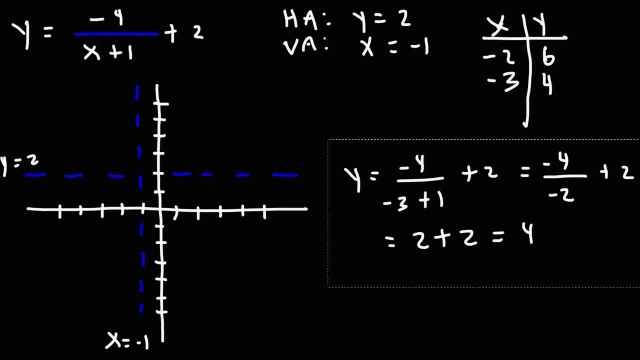 That will give us 4.. Now let's pick two points to the right of the vertical asymptote. We can try the y-intercept where x is 0 and when x is 1.. When x is 0, we get 0 plus 1, which is 1 on the bottom. 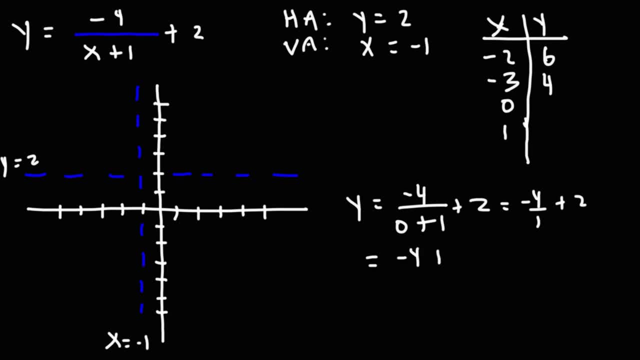 Negative 4 divided by 1 is negative 4 plus 2.. That will give us negative 2.. And if we were to plug in positive 1,, 1 plus 1 is 2.. Negative 4 divided by 2 is 2.. 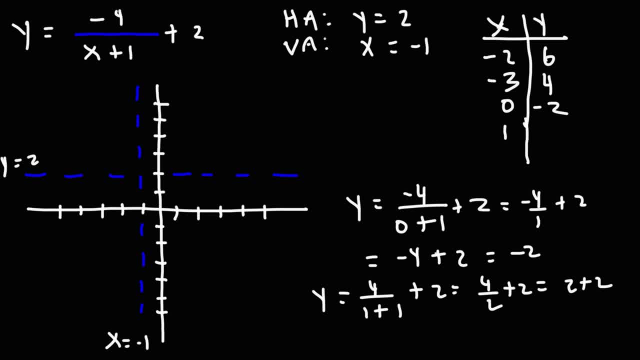 2 plus 2 is. This should be negative 4,. by the way, Negative 4 divided by 2 is negative 2.. Plus 2, that will give us 0. So that gives us the x-intercept. So, plotting the points, we have negative 2, 6.. 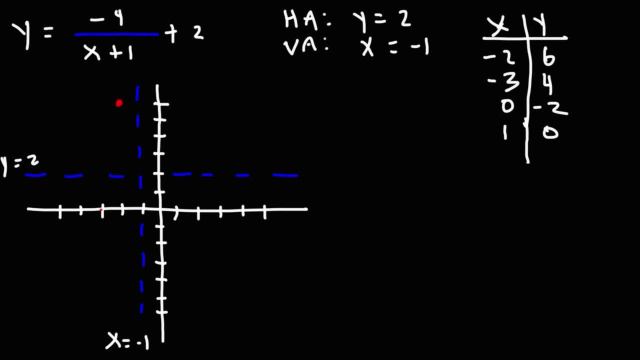 Which should be here, And then negative 3,, 4.. At 0, we have negative 2. And at 1, we have 0.. Now let's get some additional points. We don't have to do this, but 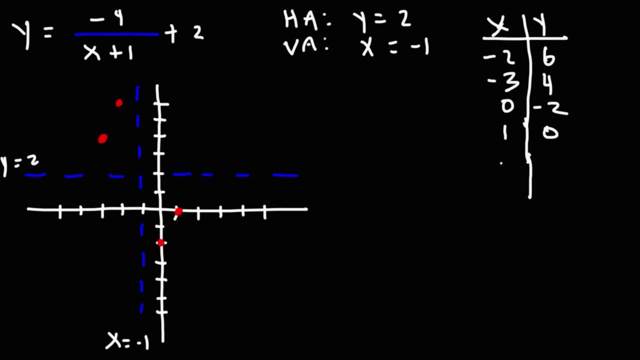 Just to make a more accurate graph, Let's pick a negative 4 and positive 2.. Let's pick a negative 4 and positive 2.. Negative 4 plus 1 is negative 3. So we have 4 over 3 plus 2..